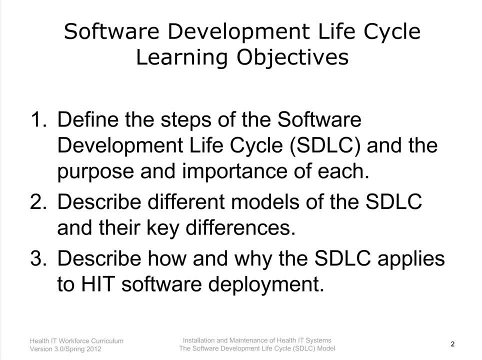 Slide 2.. The objectives for this unit are to define the steps of the Software Development Life Cycle, or SDLC, and the purpose and importance of each. Describe the steps. Describe different models of the SDLC and their key differences. Describe how and why an HIT software application would go through the SDLC. 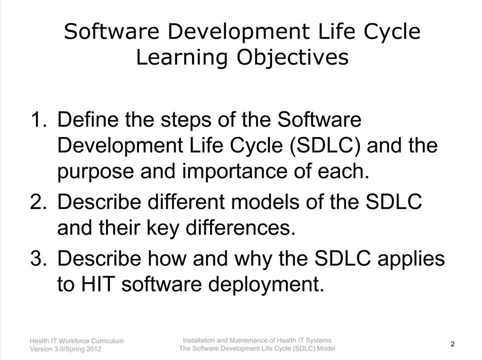 The SDLC is a well-developed concept from the IT world that promotes an organized, long-term view of the software you're working with, from its birth to its death, hence the term life cycle. It's important for those who work in health care IT to understand this model and apply it when appropriate. 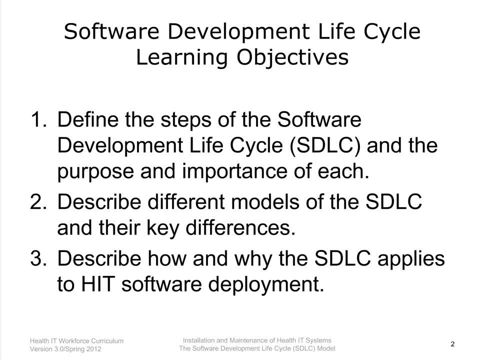 This will be crucial if you work in an institution that chooses to build its own EHR components. But even if your institution lets a commercial vendor make all the changes to the software, it will be helpful to understand the conceptual phases they are using, particularly since your institution's success will be dependent on the outcome. 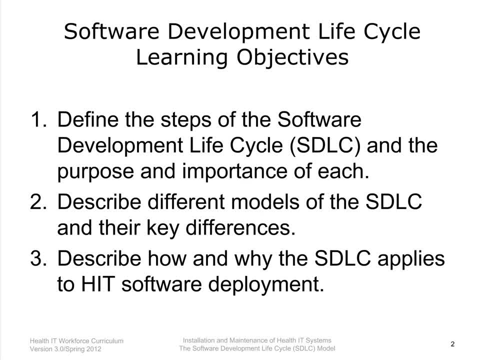 We'll start by describing the SDLC and its importance. then we'll discuss the conceptual phases of the life cycle. Then we'll look at three different models: The waterfall, iterative and spiral models that illustrate different views of the relationships between the phases. 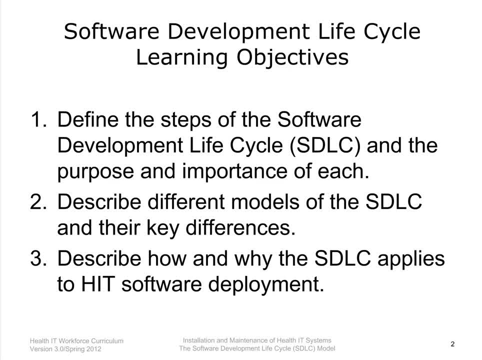 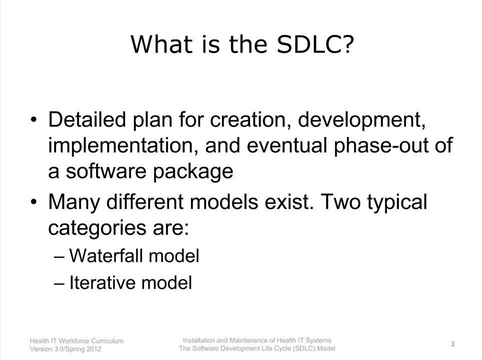 Then we'll go through an example of the SDLC in practice. Finally, we'll close with more remarks about the role of the SDLC in EHR systems, Slide 3.. The SDLC is a term used for modeling a detailed plan for the creation, development, implementation and eventual phase-out of a software. 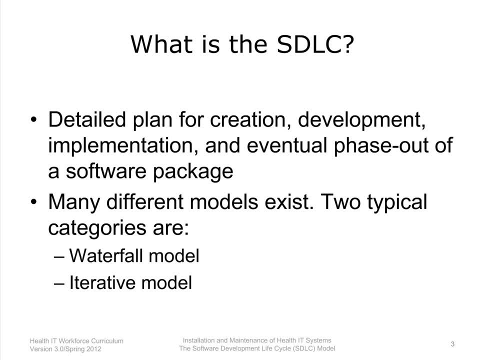 It's not about the name of the software or software system package. It's a complete plan outlining how the software will be born, raised and eventually retired from its function. Many different SDLC models exist. Each of these models was designed to fit a specific business needs, model, to accommodate available resources and skills, or to take advantage of a specific programming language or tool set that would be used. 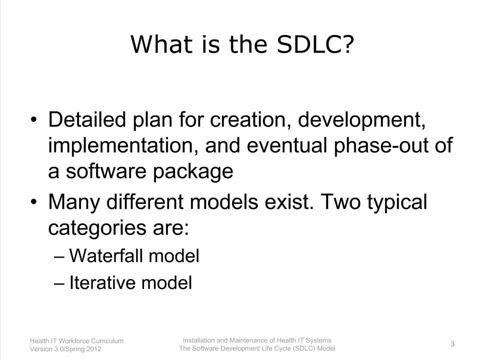 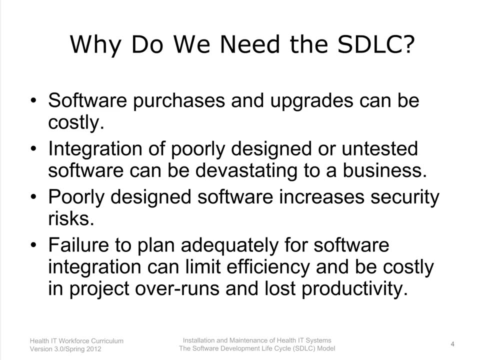 Usually, these models can be divided into two categories: the waterfall model and the iterative model, each employing a different workflow philosophy: Slide 4.. So why is SDLC important anyway? Well, as computers and software became integrated into the business environment, 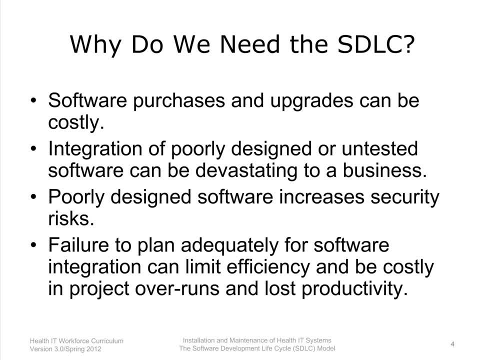 and businesses became more dependent on computers, not only to manage their business data, but also to assist or track every aspect of the workflow process. it became increasingly apparent that poor design or failure of software can be quite costly in terms of lost productivity. Additionally, poorly designed software can increase security risks and decrease data integrity. 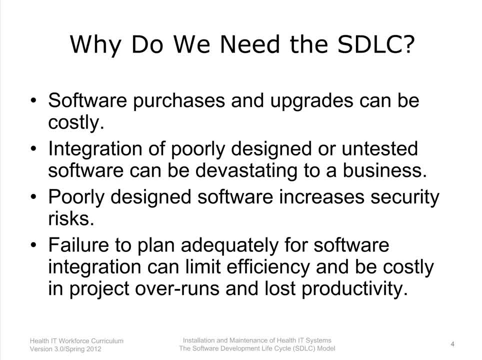 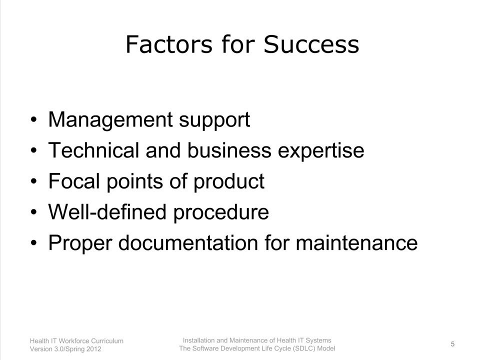 Replacement of outdated or inadequate software can cost many thousands of dollars. Therefore, SDLC was designed to control the development environment to help ensure that developers produce a high-quality system that is easy to use, and easy to use- Slide 5.. Factors for developing a successful SDLC are not unlike those already discussed in previous units. 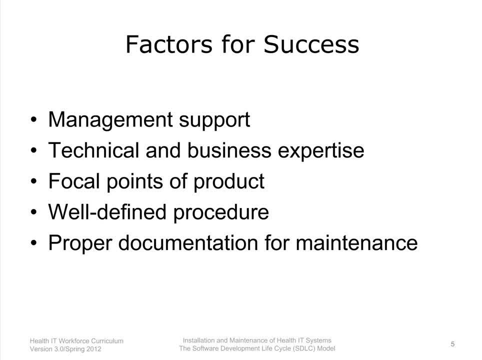 for developing your successful project plan or for selecting your EHR system. Again, these factors are not steps in your SDLC. Rather, they are elements that will dictate whether the SDLC will be followed, which, in turn assures the success of the program being developed. 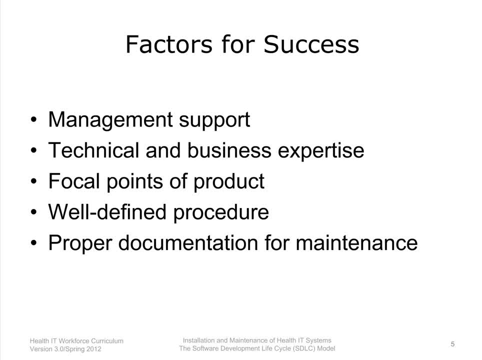 Developers need to have the support of the management as much as possible, since management will dictate, the business need budgeting and top-level buy-in for the product. Technical and business expertise. As in any field, there are experts, in this case, programmers. 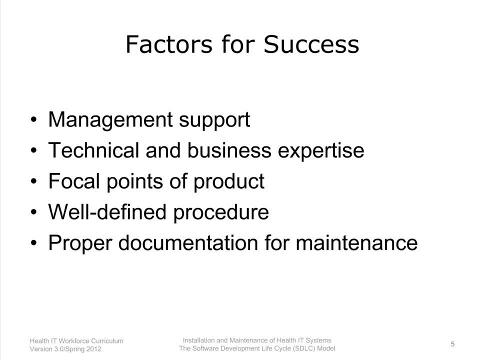 who just know what needs to be accomplished, even when the objective is originally presented. These programmers know which SDLC model is most appropriate for the programming language or toolkits that need to be utilized to ensure the software project will be successful. Likewise, business experts are also critical in the software development cycle. 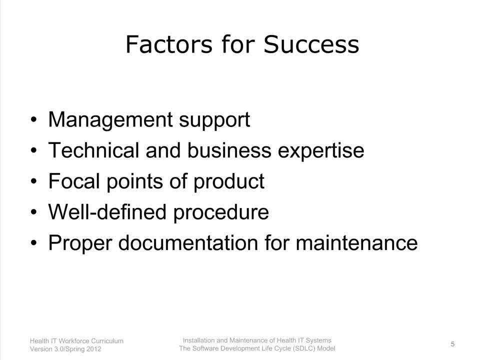 since they understand the overall demand and needed functionality for a particular software. Additionally, business experts can help determine whether the software will eventually show any cost savings over other products or processes, Determining the product focal points. Some parts of the program should be rated a higher priority than other parts. 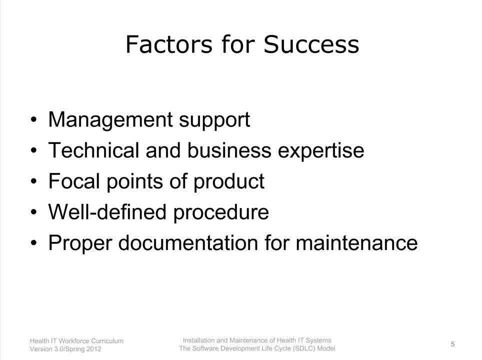 Choosing which elements are most important will allow developers to make decisions when issues arise which may compromise the software's overall functionality, ensuring that there will always be some strong. strong selling points in the developed software, compared to a product that provides only mediocre service. Follow well-defined procedures. 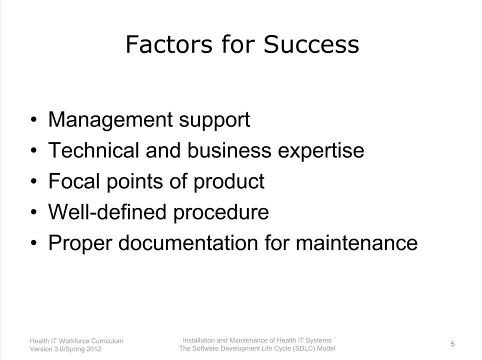 Developers should have a clear understanding of goals at each phase, along with the methods and accepted tolerances for evaluating each of the goals. Develop proper documentation for maintenance. Developing good documentation will help with the implementation and continued success of the product throughout its implementation. 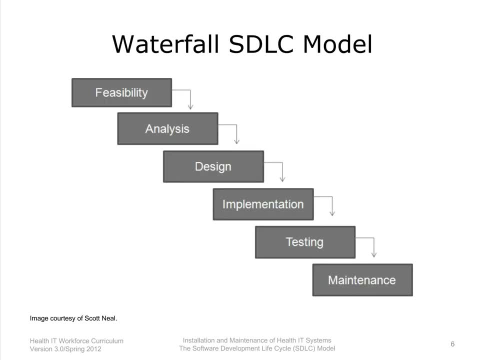 entire life cycle, Slide 6.. Now let's take a brief look at how these phases can relate to each other. initially, using the so-called waterfall model, The initial assessment of feasibility is followed by an analysis phase, which is followed by the design phase, which is followed by the implementation phase, then the testing phase. 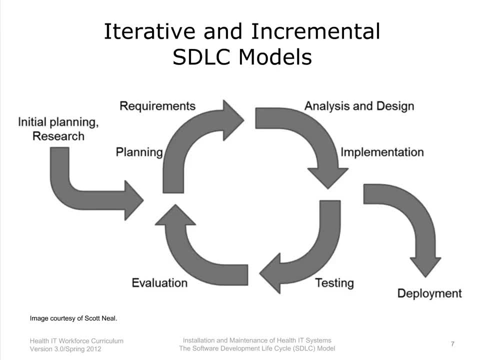 then the maintenance phase, Slide 7.. Interpret that with this iterative or incremental model, which starts with initial planning and research, then begins a cycle consisting of planning requirements, analysis and design, implementation, testing and evaluation, which repeats as needed until the decision is made. 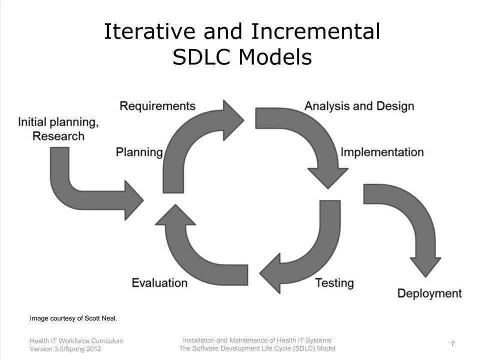 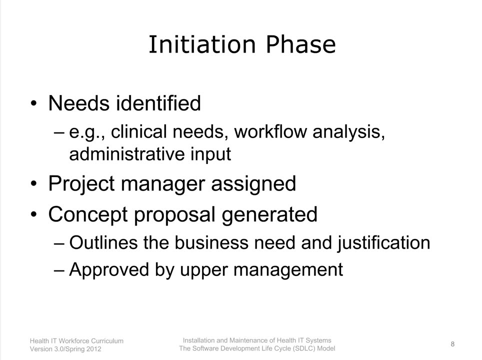 to do deployment. We'll discuss the models in more detail at the end of this unit. Now let's discuss what each phase generally entails. Slide 8. Initiation In the software vendor world, where profits are realized by fulfilling consumer market. 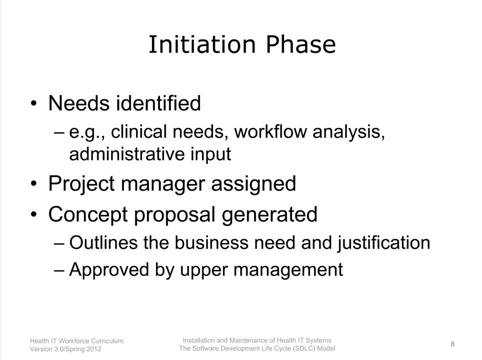 needs with new software products. initiation is where a need is identified for a new software system. Software development companies use this stage to determine the needs of the present market. The software vendor's management is often involved in this stage, as they want to determine. 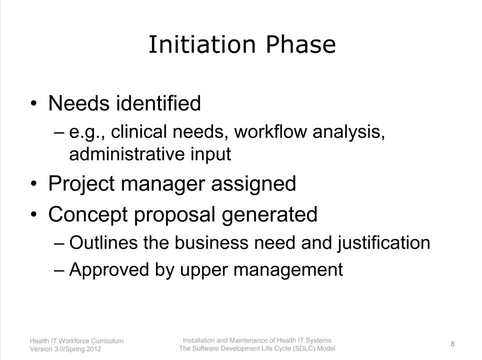 what the developers have to do and how it will impact the market- Slide 8.. In a clinic or other healthcare institution, this need is usually identified by clinicians or staff, such as a flawed workflow process or other issue. For instance, a healthcare clinic currently uses three different programs to record patient. 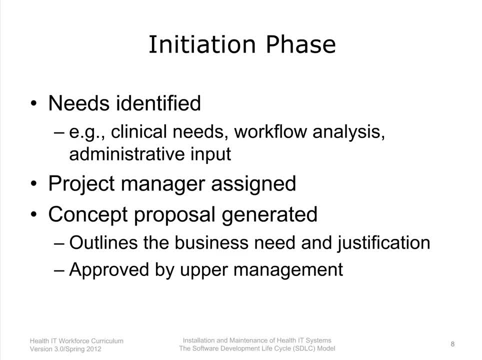 data, dispense online prescriptions and run the business office, requiring a lot of work, overlap and generation of paper documentation between systems. Both the physicians and the billing department are looking for additional support for the clients and they are looking for more efficient ways to communicate and improve efficiency. 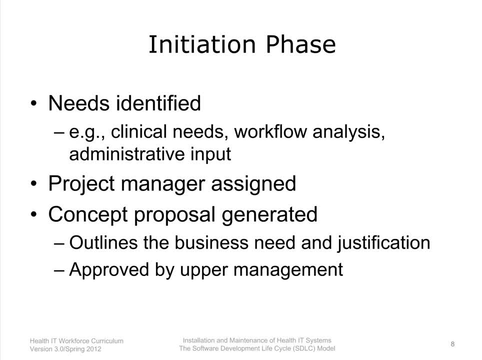 They would like a system that can communicate seamlessly between the various business components and streamline operations- Slide 9. A project manager typically would be assigned and would eventually generate a concept proposal, a document which identifies the problem and why the new system needs to be pursued. 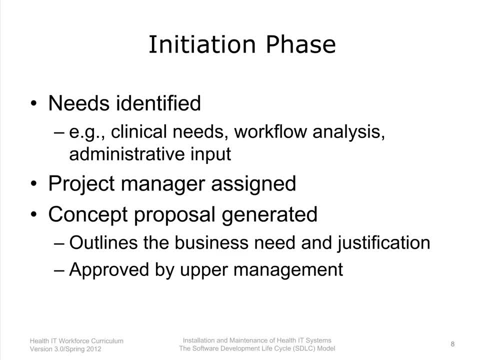 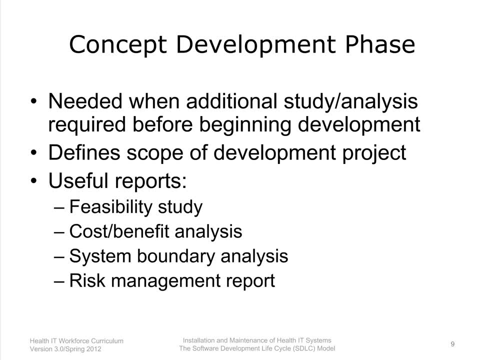 Upper management would then review the proposal and approve it, and the project moves on to the next phase, Slide 10.. The concept development phase begins when the concept proposal has been formally approved, but when additional study and analysis are required prior to system development activities. 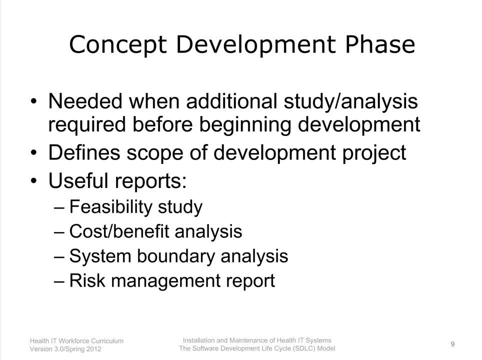 We begin to analyze what will be necessary to complete the project. Here all relevant factors are analyzed to develop the project scope. Several reports can be created here. Feasibility study, In other words, will it work? Slide 11. cost-benefit analysis, in other words, is the cost really worth it? system boundary. 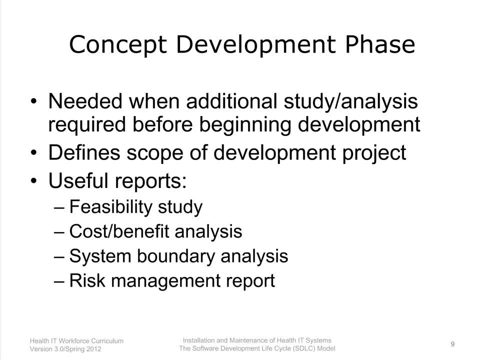 in other words, how far should the project go. risk management, in other words, what will happen if we don't do it? these reports are then presented to the powers that be and a decision is made whether or not to go ahead. they approve the funding. if they give their approval, it's on to the next phase. 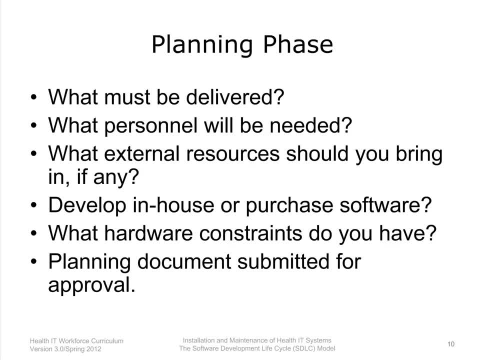 slide 10. during the planning phase, we determine who is doing what, when and how, along with the personnel and other resources that will be needed to complete the project. for instance, should we use existing personnel or hire consultants. during this phase, we determine what developmental resources will be required. 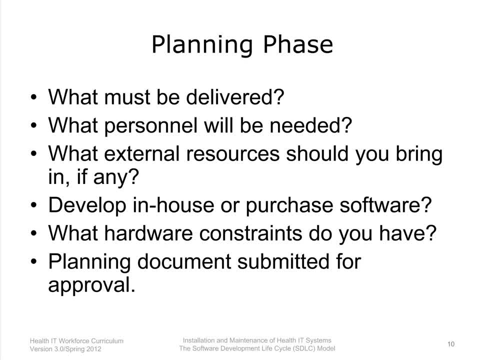 to create the specific software. other questions are also contemplated during this phase. should we develop in-house software or you, or buy it off the shelf? what are the deliverables, such as completed software, programming and documentation, user manual training, testing plans, et cetera? finally, a planning document is submitted to management. 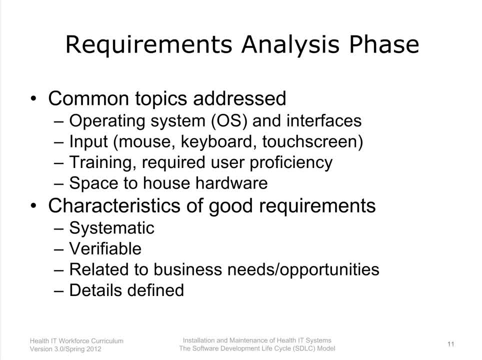 for approval: slide 11: the requirements analysis phase focuses on what the system will do, in an effort that considers all stakeholders, including sponsors and potential users, as important sources of information. during this phase, you will determine what operating system or OS and interfaces are required. for example, will it run? 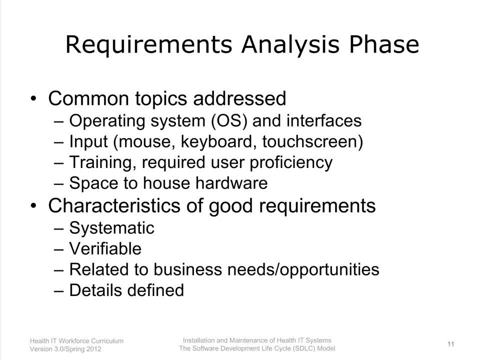 with Windows or Linux. here you will answer a number of other questions as well. what functionality will be required? should be run with the mouse, keyboard or touchscreen input? how much training will be required of the user? will a new room be needed for the hardware that runs the system? 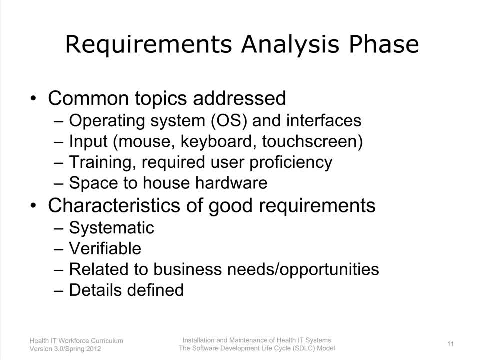 slide 12. there are a variety of techniques that can be used to gather the requirements, but some key points to remember are that the requirements must be systematic, verifiable, related to identified business needs or opportunities, and defined to a level of detail sufficient for system design. once the requirements documentation is approved, the project moves on to the 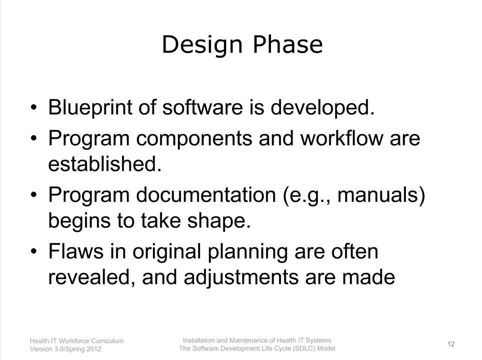 design phase, slide 12. the design phase takes those requirements and develops a deep, detailed blueprint outlining the software specifications. here the program architecture, which defines the various software components along with their interfaces and behaviors, is established. the design phase is also where much of the program documentation begins to take shape, including the maintenance manual. 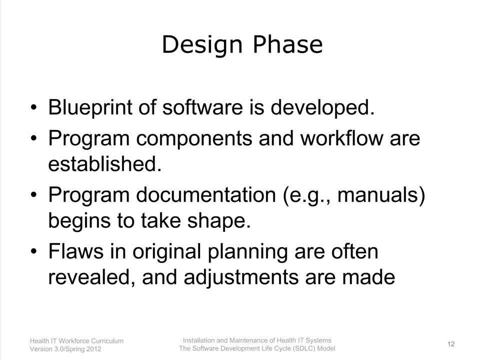 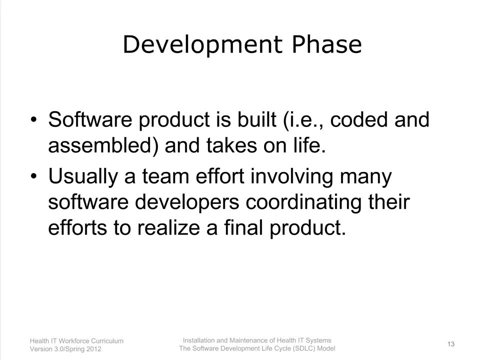 operations manual and training manual. flaws in the original planning which require some adjustment are often revealed during the design phase. slide 13: the system is built during the development phase. this includes source code files, header files, make files and binaries. this is where everything is coded and assembled and the actual design of the 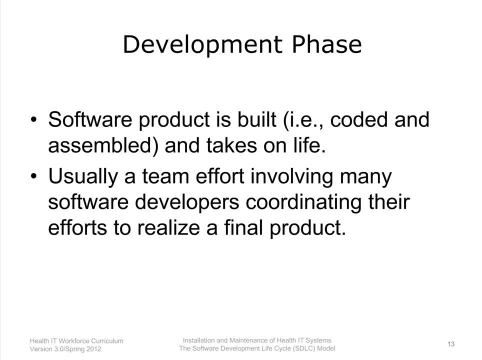 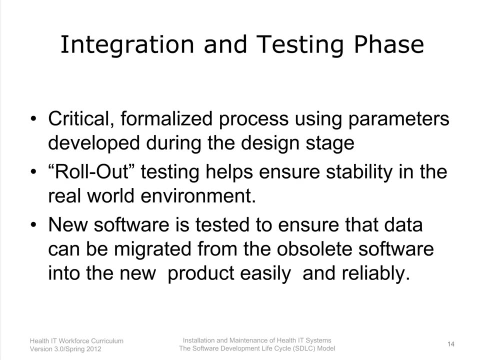 system is realized as living, breathing software. this process is usually a team effort with its own set of sub goals and milestones, involving many software developers who coordinate their efforts to a final product. slide 14: integration and testing of the entire system is a formal, documented testing procedure which ensures that the system performs as designed, testing the rollout of the 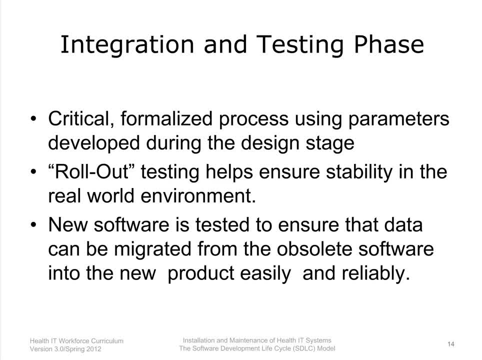 system also begins including migration of existing data into the new system, as well as usability. usually the system is rolled out over a weekend so that if anything goes wrong, the old system is still active and available. integration and testing is a critical step. if the software fails testing, 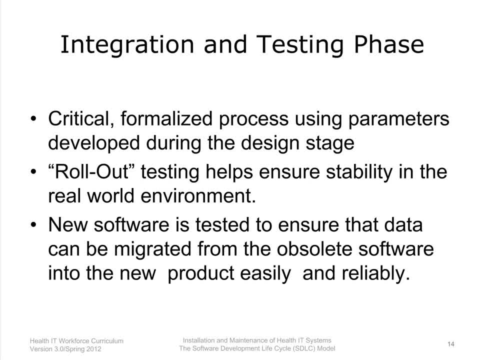 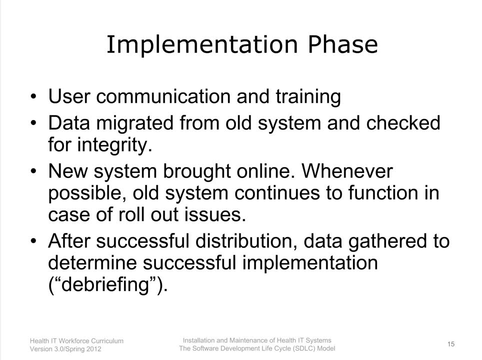 it cannot be trusted to work. approval of testing and test results is necessary before the project moves into the next phase- implementation slide 15. now that the software has been formally tested and passed, it is time for distribution to the production environment. in this implementation phase, user training and testing is required to ensure that the software is tested and tested. 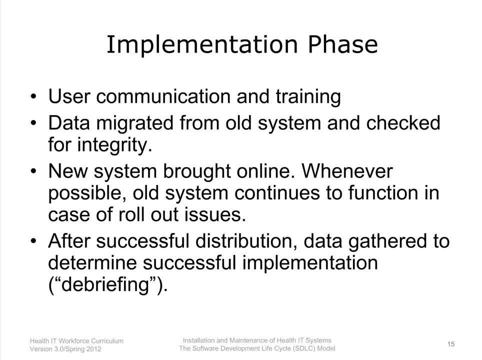 training takes place, previous data is migrated and the system is brought online. after the system goes live, it is once again tested and data is collected to determine if it is working to specifications. this process is often referred to as a debriefing. it is also where any problems that 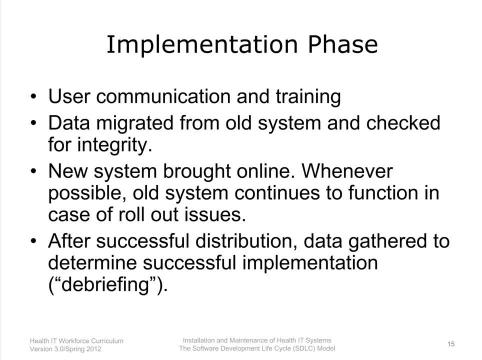 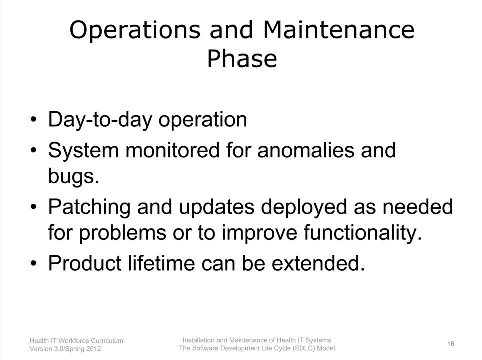 were not crucial to the implementation can be addressed and any necessary changes to the system documented for future versions. slide 15. slide 16: the operations and maintenance phase is the day-to-day operation of the software. after deployment, the software must be maintained, patched and regularly updated to ensure long, reliable life. 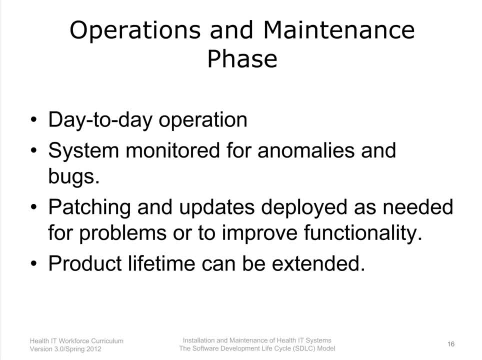 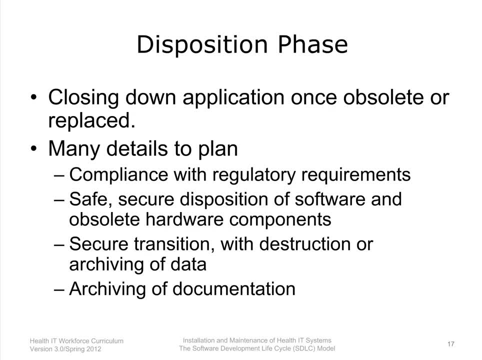 upgrades can be tested and deployed to improve functionality. slide 17: every software application eventually becomes obsolete. perhaps a new system is being developed or this system cannot keep up. whatever the reason, disposition involves more than just shutting off the server. often the system may be kept going due to regulatory requirements or because there are still. 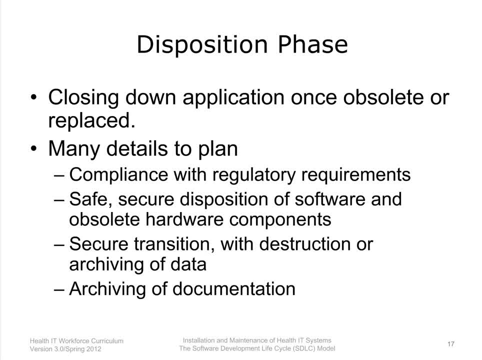 projects using it. sometimes there is data on board that must be kept safe and secure even after its useful life is over. software disposition needs to be planned to ensure that you meet all regulatory requirements and ensure a smooth transition between the system and the software project. whatever the replacement product will be, A disposition plan must be developed. 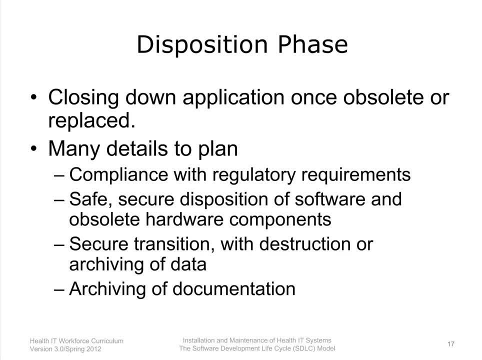 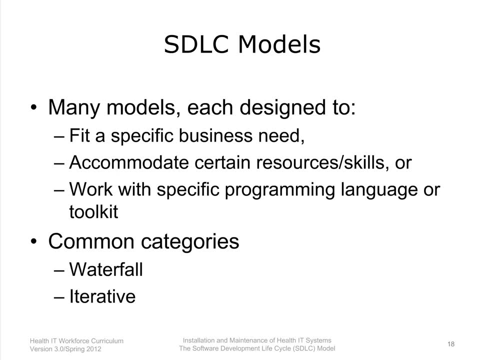 which may outline everything from the dismantling of the software itself to the safe and secure disposal of old hardware and data, to archiving of documentation- Slide 18.. As briefly shown and discussed earlier in this presentation, many different SDLC models exist. Each of these models was designed to fit 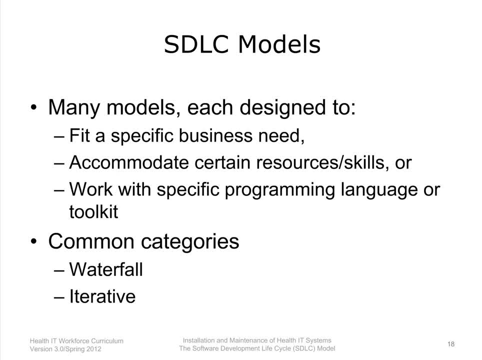 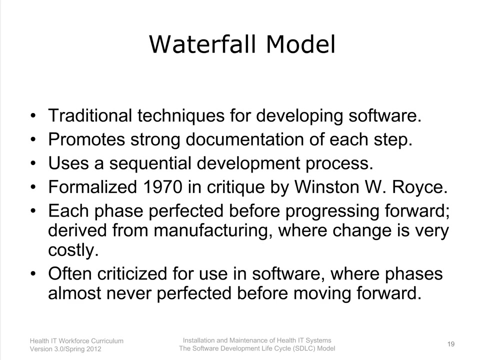 specific business needs, to accommodate available resources and skills or to work with a specific programming language or toolkit. Usually, these models are divided into two categories: the waterfall model and the iterative model, each of which employs a different workflow philosophy- Slide 19.. The waterfall model uses more traditional planning, testing and 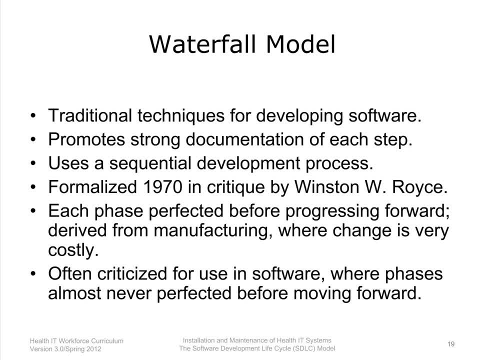 implementation techniques to design and implement new software products. This model promotes strong documentation of each step of the development process. The waterfall SDLC model represents a sequential development process where progress is seen as flowing steadily downwards through each of the phases of development. Winston W Royce has been 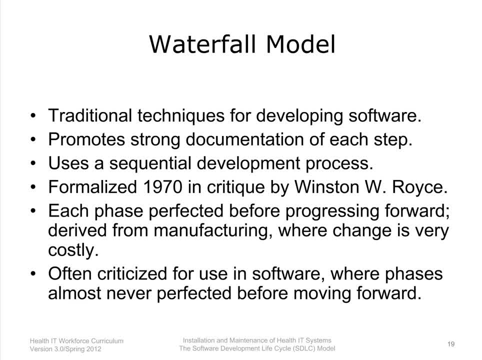 given credit for formalizing the waterfall model in an article around 1970 where he presented this modeling concept as flawed from a software development standpoint- Slide 20.. The waterfall development model is actually a product of the manufacturing and development industries, where making after-the-fact changes is often. 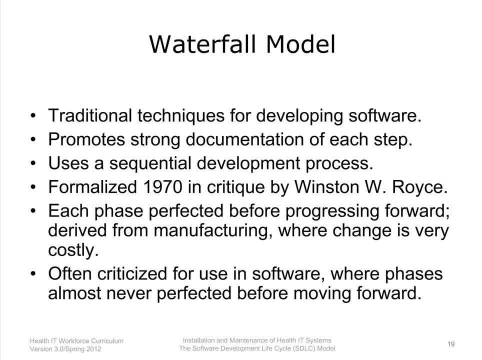 prohibitively costly. Therefore, progression to the next phase of development does not typically commence until the previous phase has been perfected and locked down. Slide 21.. Many have criticized the waterfall model, citing that it is difficult, if not impossible, to finish a phase of a software product's lifecycle perfectly. 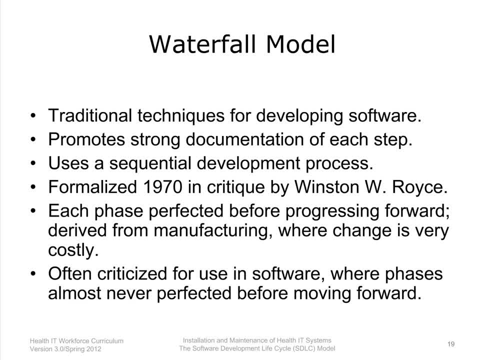 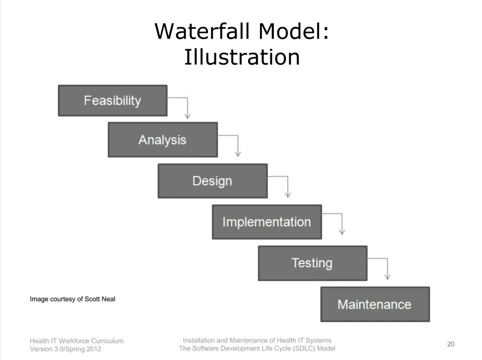 before progressing forward. To that end, several variations of the waterfall model have been created to help address some of these issues. Slide 20. This diagram, which I described on an earlier slide, depicts just one of the many variations of the waterfall model employed by developers. As this variation of the waterfall 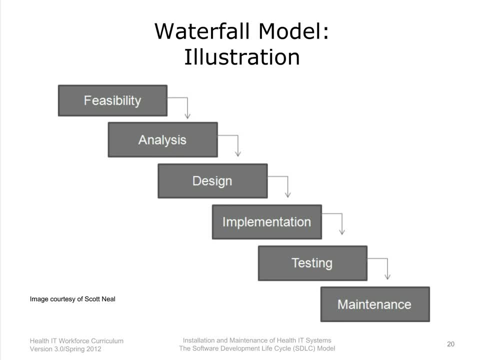 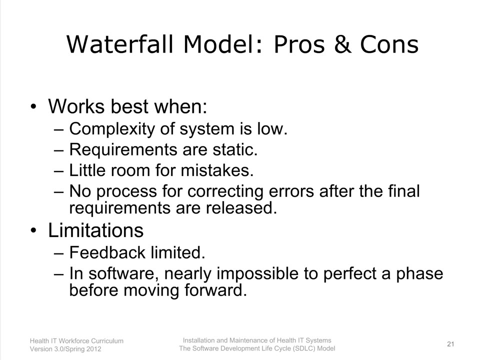 model suggests. the waterfall model can best be described as a sequential software development process whose overall development process is based on the development of a software whose workflow progresses in a linear downward fashion, just like a waterfall flows- Slide 21.. Using a waterfall methodology is most likely to be successful when the complexity 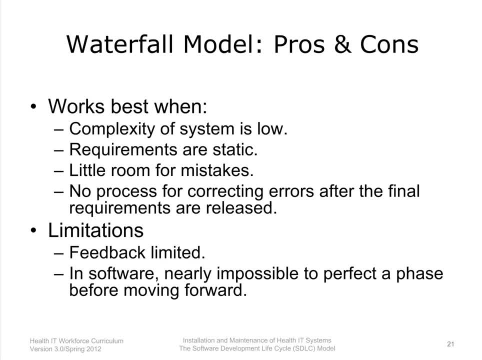 of the system is low and requirements are static, but there is little room for mistakes and no process for correcting errors after the final requirements are released. Feedback can be quite limited when using this approach and, as I mentioned previously, there is no fixed limit on the progress of the process. Slide 22.. The waterfall model is a very important graphic model which provides an opportunity for developers to practice their own models. When the process is completed, the model is gradually forfeited to the kids and other students. As I said previously, most believe 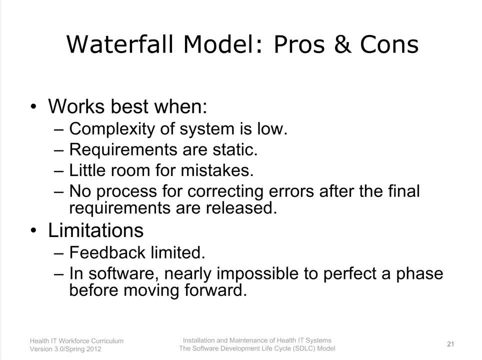 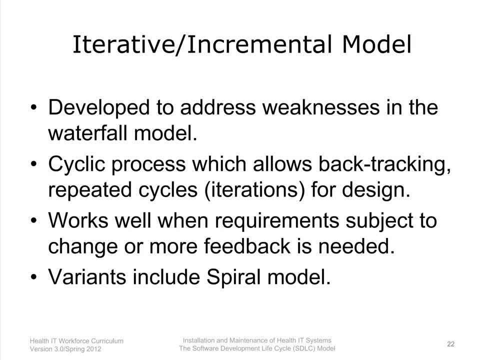 it is nearly impossible to finish a phase of a software product's lifecycle perfectly before progressing forward to the next stage- Slide 22.. Iterative and incremental model. These models were developed in response to identified weaknesses of the waterfall model and often considered cyclical in nature. 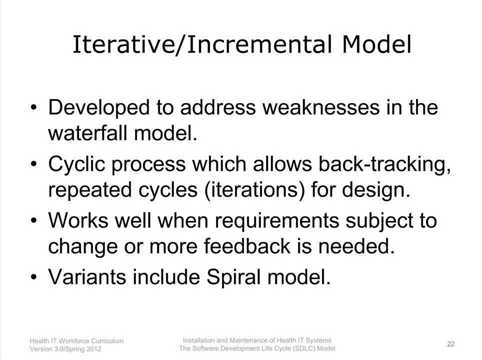 One variation of the iterative model is the spiral model, which we will look at after we see a more basic iterative model. This approach works well in environments where perceived requirements are subject to change as the project progresses or where more feedback is warranted. Let's take another look at the illustration. 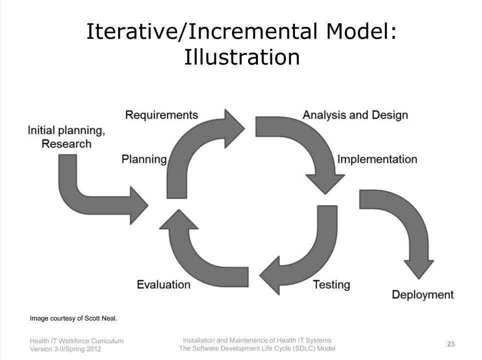 Slide 23.. As you can see from this diagram, which I described earlier in the presentation in iterative models, the phases of software development take on a more cyclical nature. It starts with an initial planning phase and ends with deployment, with the cyclic interactions. 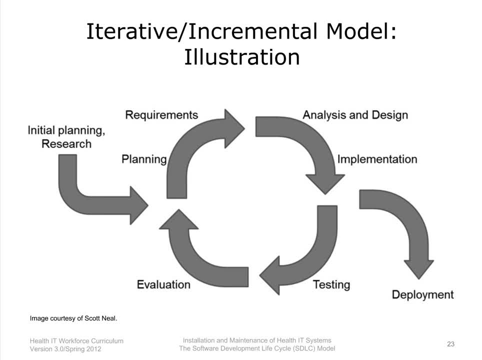 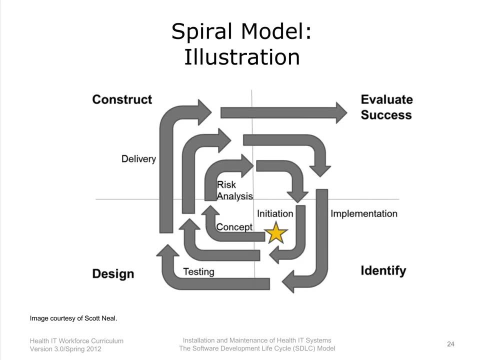 in between or even after the initial deployment occurs. With this model, several deployment cycles of the product are possible as the software becomes further refined, analyzed and tested and as new enhancements are added- Slide 24.. Another variation of the cyclical model is the spiral life cycle or spiral development. 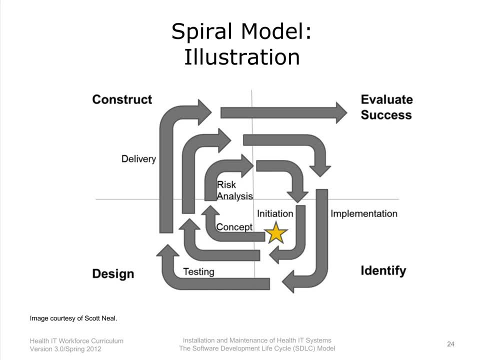 model. This model combines the features of another model called the prototyping model with those of the waterfall model. The spiral model is intended for large, expensive and complicated projects where client responsiveness is a significant issue. In this model, one or several prototypes may be created throughout the life cycle. 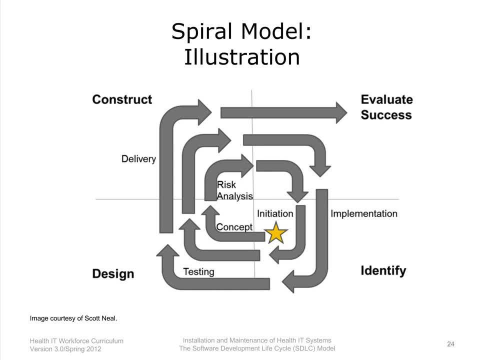 At each iteration, the prototype is tested and further input is gathered until all concerns have been adequately addressed. Let's walk through the diagram. The action begins in the center of the spiral with initiation and then cycles repeatedly through four conceptual quadrants – identify, design, construct and evaluate. 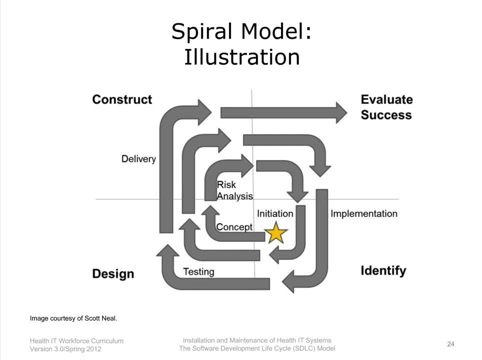 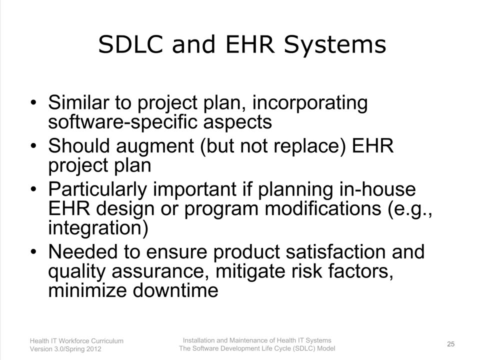 The first cycle contains the phases concept and risk analysis. Later cycles contain the phases implementation, testing and delivery, Slide 25.. As you can see, the SDLC is very similar to a project plan, but it integrates several software-specific aspects into the planning infrastructure. 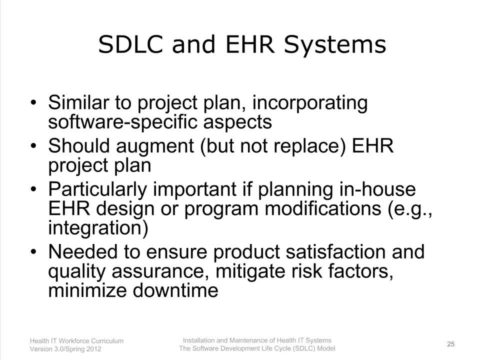 to specifically address the concerns associated with developing and deploying a new software system. However, you should consider an SDLC as augmenting your overall EHR project plan, not replacing it. Employing SDLC in your environment when developing a new EHR system. 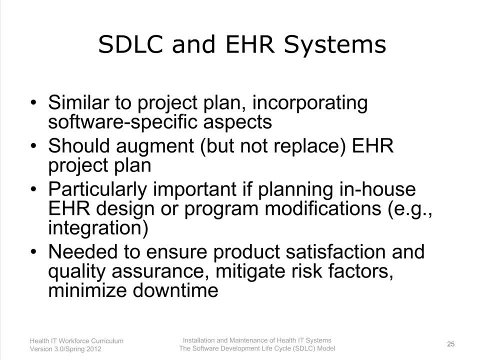 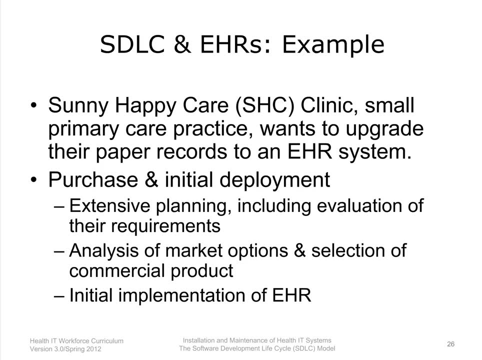 or designing changes to an existing system is crucial to ensuring that your new software, whether developed in-house or purchased off-the-shelf, adequately meets expectations while mitigating overall risk to the organization- Slide 26.. Now let's discuss a scenario in which EHR installation utilizes 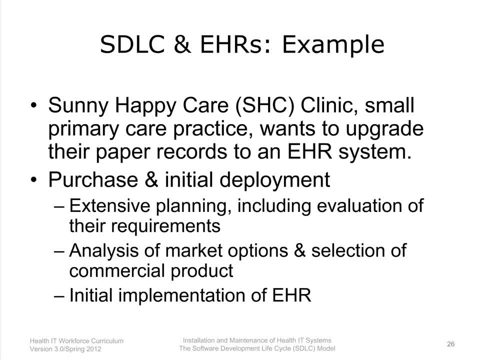 SDLC-based software for development. SDLC Principles. Sunny Happy Care SHC Clinic, a small primary care practice, wants to upgrade their paper records to an EHR system. Before purchasing and deploying, they do extensive planning, including evaluation of their requirements and analysis of market options. 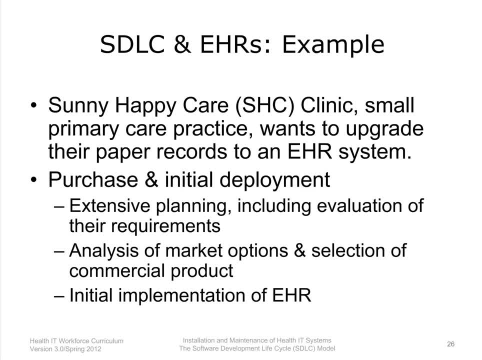 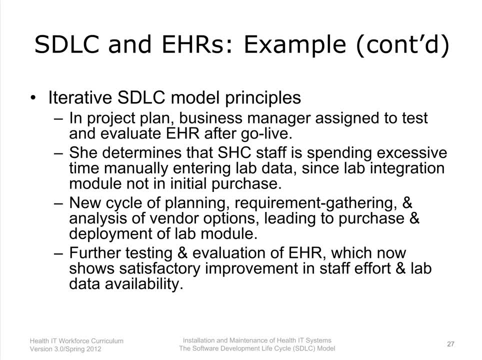 They ultimately select and implement a commercial EHR, Slide 27.. You'll have to be very careful when you're developing a new EHR system. You'll have recognized those actions by the clinic staff as several of the general steps in the SDLC. 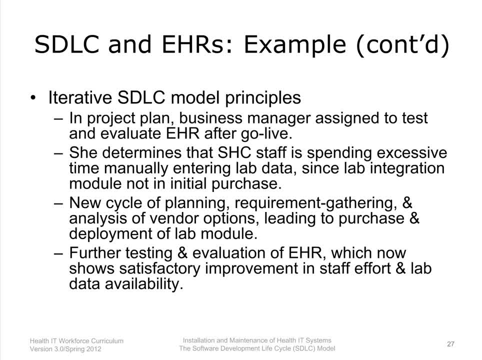 The fact that they are specifically following an iterative SDLC model in their deployment soon becomes clear. According to the project plan, the business manager has been assigned to test and evaluate the EHR after go-live. In her analysis, she determines that the SHC clinic staff is spending excessive time. 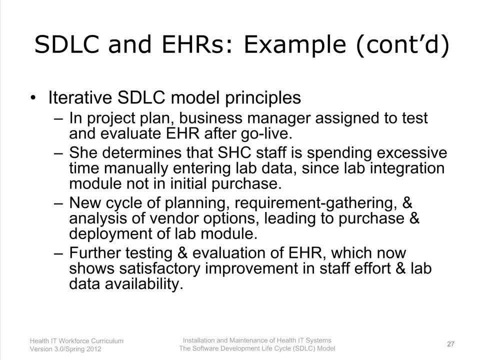 manually entering laboratory data: Slide 28.. You'll have to be very careful when you're developing a new EHR system, Since a laboratory integration module was not part of the initial purchase. Thus, the staff enters a new cycle of planning: requirement gathering. 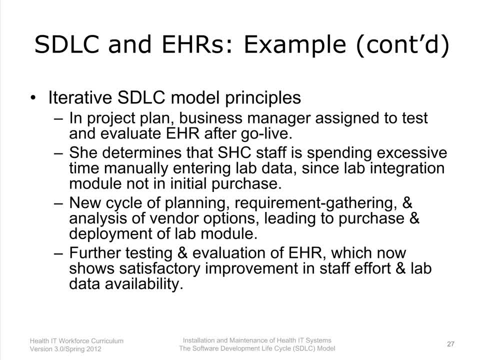 and analysis of vendor options leading to purchase and deployment of a laboratory module. Subsequent retesting and re-evaluation of the EHR now shows satisfactory improvement in staff effort and availability of lab data- Slide 28.. This concludes our unit on the software development lifecycle. 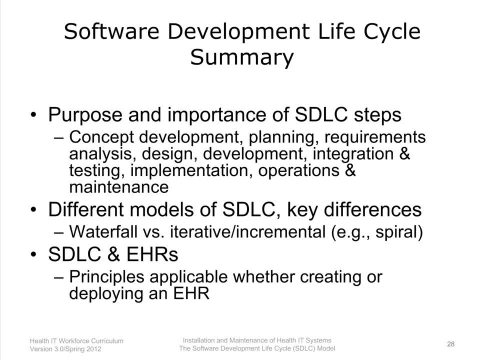 In summary, the SDLC is a set of steps that were codified by the software development industry but are useful in executing many types of projects. Common steps include concept development, planning, requirements, analysis, design, development, integration and testing, implementation, and operations and maintenance. 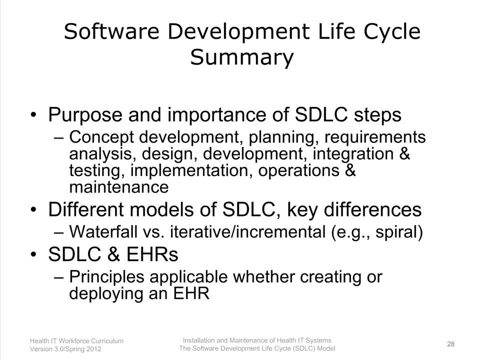 Slide 29.. The relationships backslidden- Slide 30.. Slide 41.. between these steps have been formulated into different models based on different needs. The waterfall is one such prominent model and it emphasizes steady progress through the steps and careful completion of each before moving on. The iterative or incremental is another.